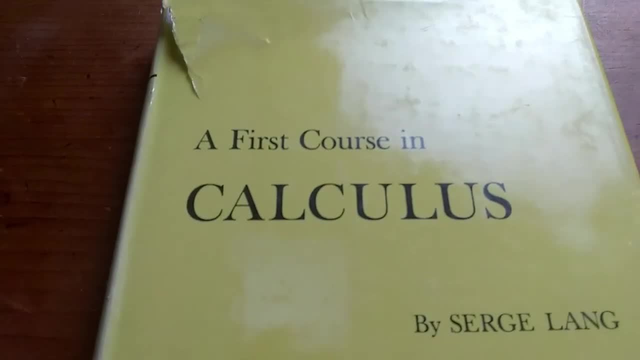 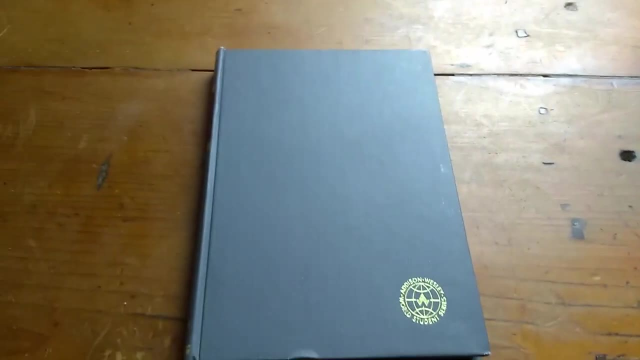 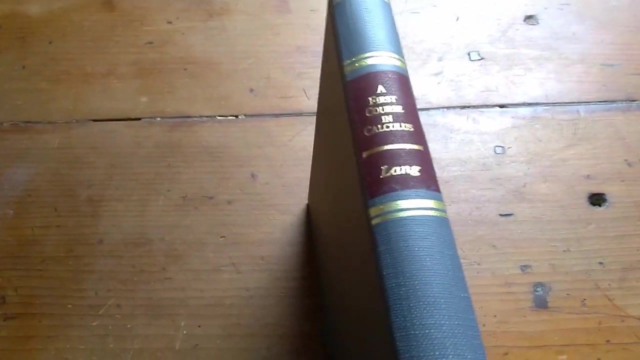 Even the name implies that: A First Course in Calculus. I have so many good things to say about this book, Let's take a look inside it. So before we look inside the book, let me show you what the cover looks like without the dust jacket. So it's got really elegant writing. See, there it says A First Course in Calculus by Lang. 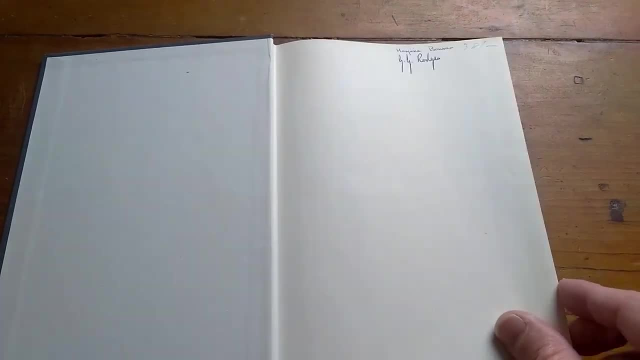 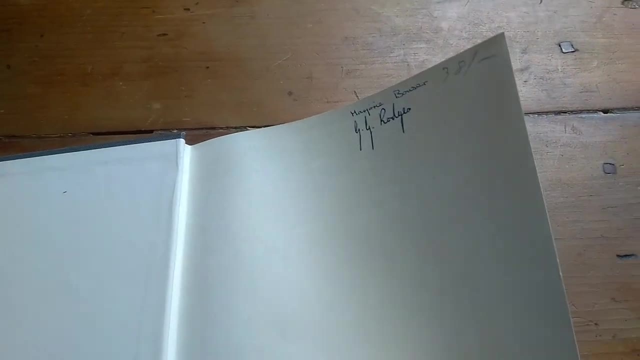 Let's take a look inside this book. It's signed there by someone. I don't know if we can make that out. 381, that's either a date or a price. One of the two. First Course in Calculus. 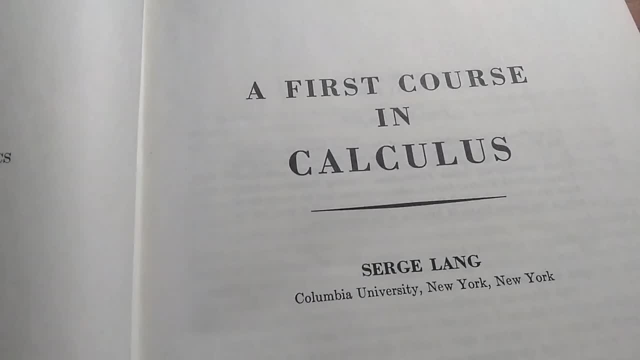 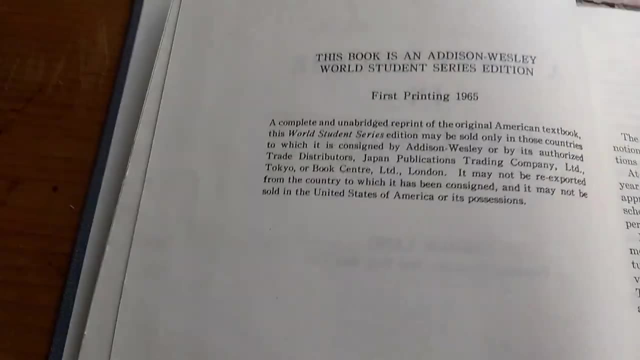 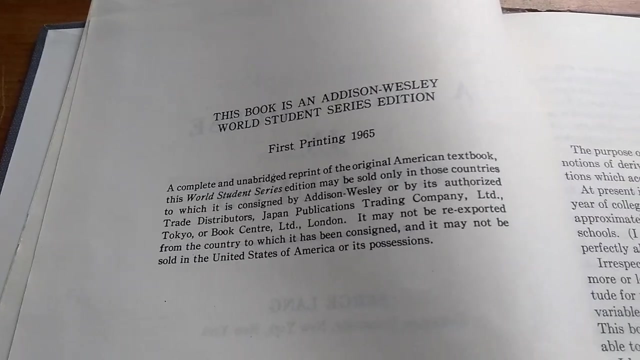 That's part of the Addison-Wesley series in mathematics, Serge Lang, Columbia University, New York, New York, With supplementary exercises. And here we go. Here is the date of the book: First printing: 1965.. Wow. 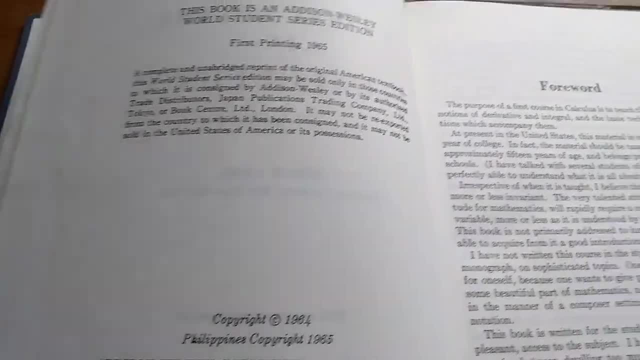 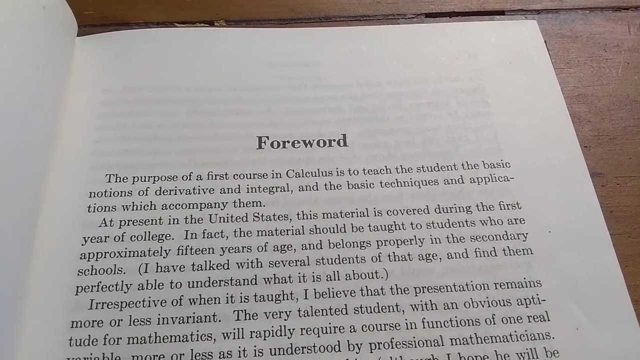 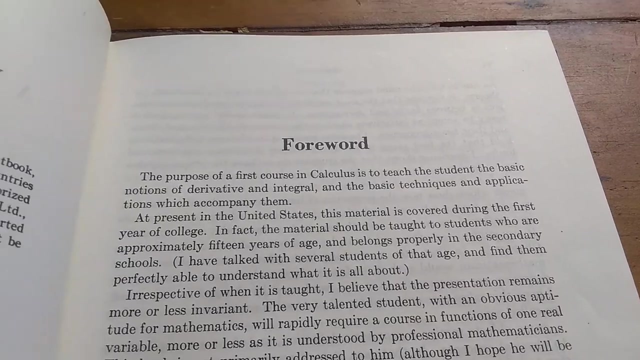 That was a long time ago, right? A very, very long time ago. And here is a forward. It says: the purpose of the first course in calculus is to teach the students the basic notions of derivative and integral and the basic techniques and applications which accompany them. Right, so this is an old-school introductory textbook. 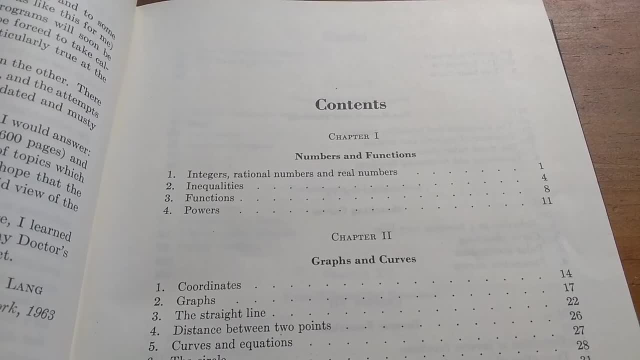 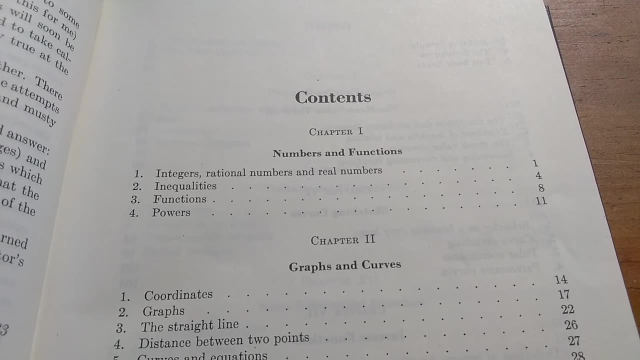 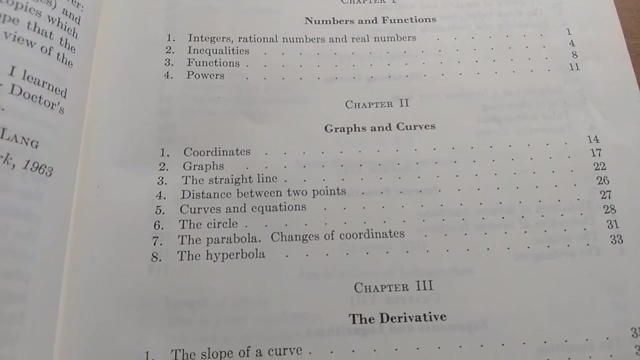 Let's take a look at the table of contents. So chapter one starts off in the very beginning: Numbers and functions. He talks about integers, rational numbers and real numbers, Inequalities, functions, crítiques etc. and powers. Then he goes on and talks about graphs and curves. Notice he. 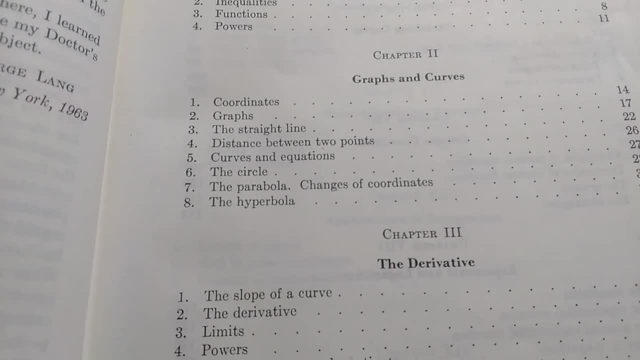 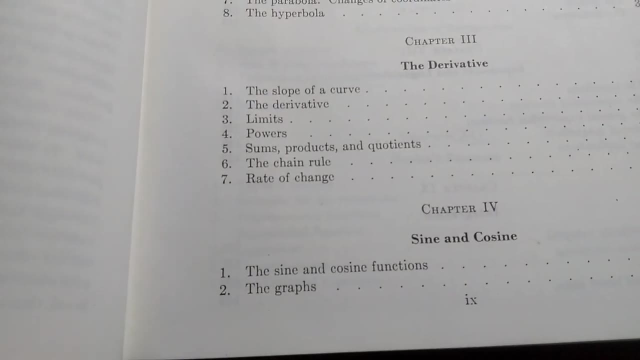 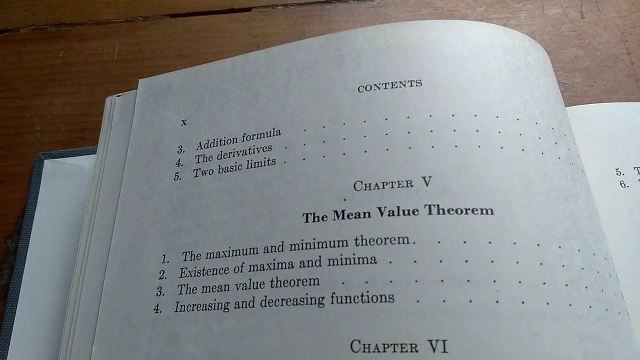 talks about parabolas and hyperbolas. This is very different from what you see in mainstream calculus books today. Then the derivative: an entire chapter on sine and cosine. He talks about the addition formula, then the derivatives and two basic limits. Chapter 5 is on the all-important mean-value theorem. Then 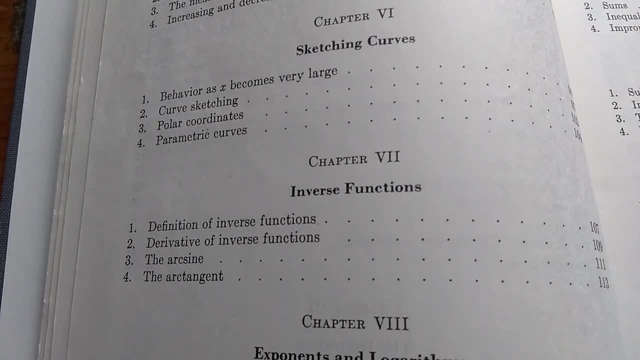 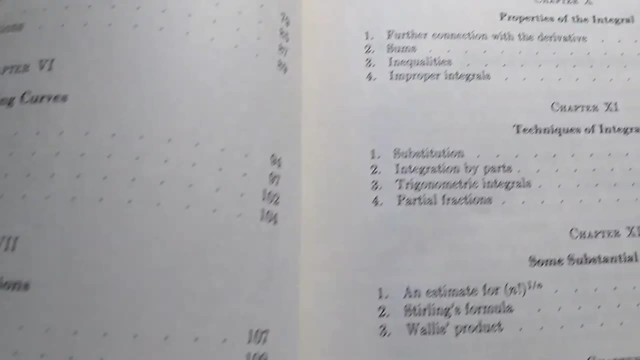 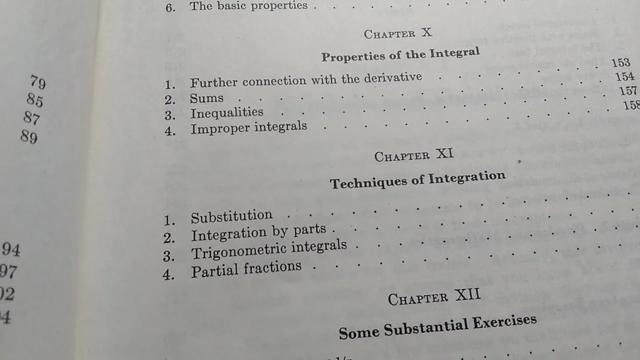 talks about sketching curves, inverse functions, exponents and logarithms, integration- going a little bit faster here- properties of the integral, techniques of integration- So it looks like he does substitution parts, trig, integrals and partial fractions, Then some substantial exercises. 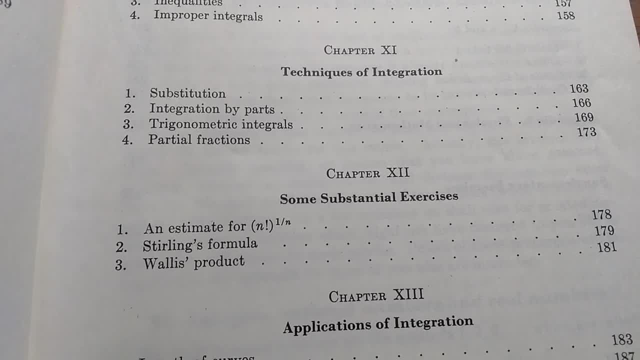 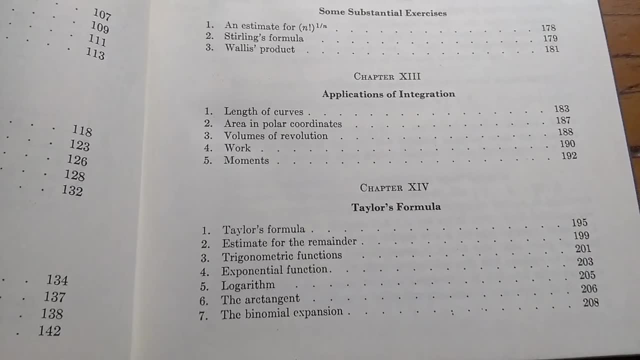 I like the name of that chapter. I mean, who does that Calls a chapter some substantial exercises? Well, Serge Lang does, that's who. And then we keep going. Then it looks like he finishes with series, which I kind of like. I finish my. 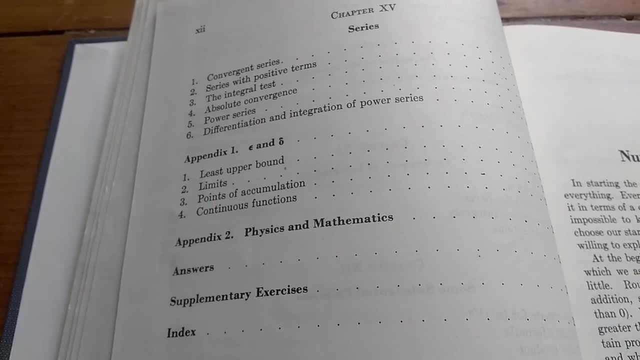 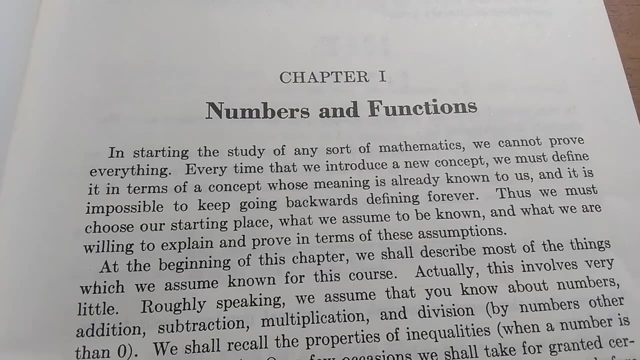 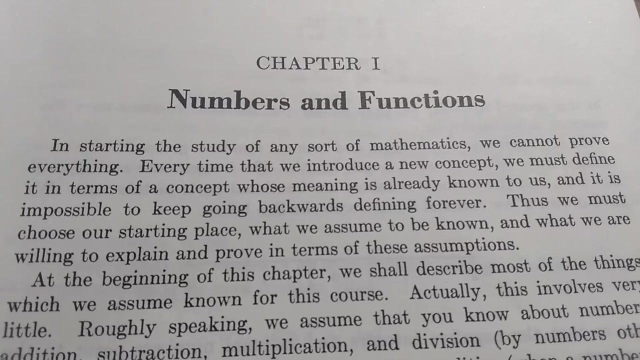 calculus 2 course with series whenever I do teach calculus 2.. I like to save the best for last and I do love infinite series. This is chapter 1.. It's called numbers and functions. Let's read it together. In starting the study of any sort of mathematics, we 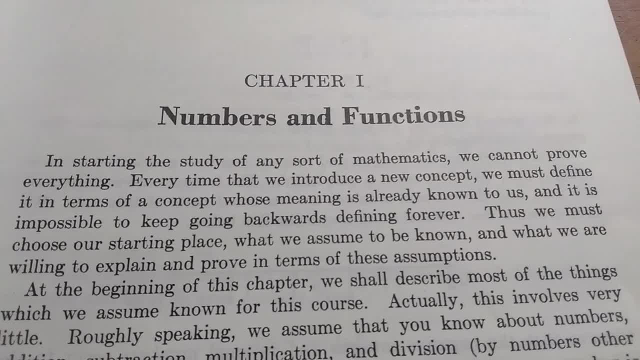 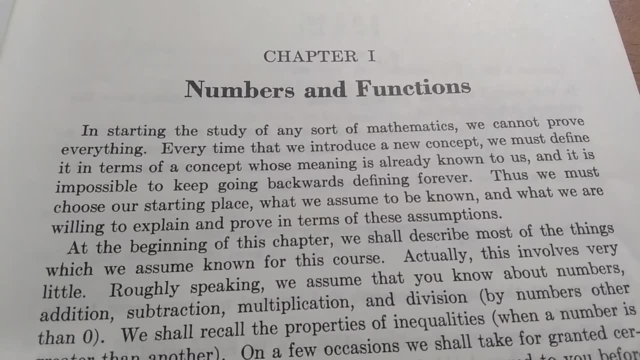 cannot prove everything. I agree. Every time that we introduce a new concept, we must define it in terms of a concept whose meaning is already known to us, and it is impossible to keep going backwards, defining forever. Right, You have to take some things for granted when you're studying math, especially the higher you 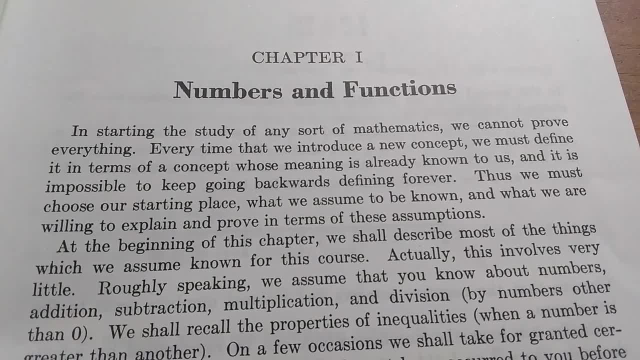 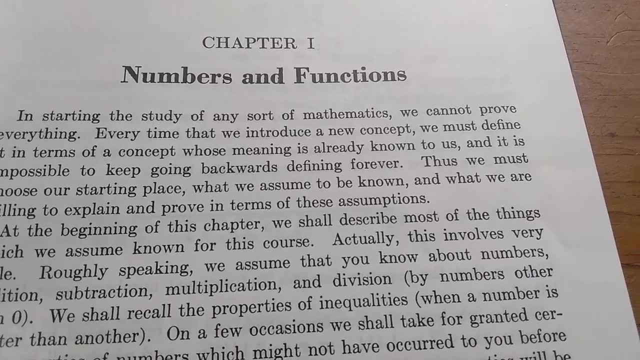 go. You know the higher you go you have to take a lot of stuff for granted that you may not know how to prove. You just assume it's true because someone else is done it before you and then you move forward. Then we must choose our starting. 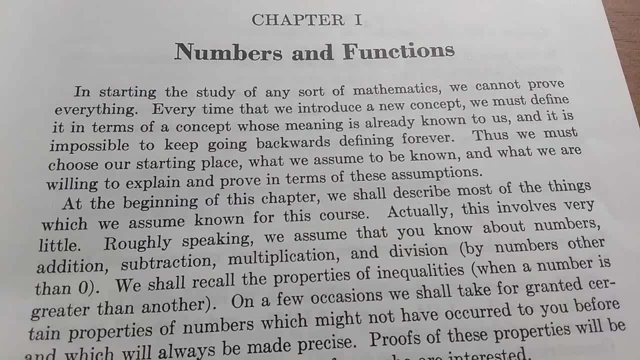 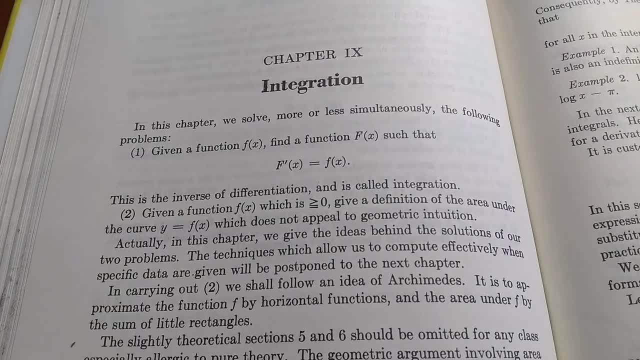 place what we assume to be known and what we are willing to explain and prove in terms of these assumptions. Very good, Mr Lang. This is the chapter on integration and the first thing I noticed when I opened it to this page. 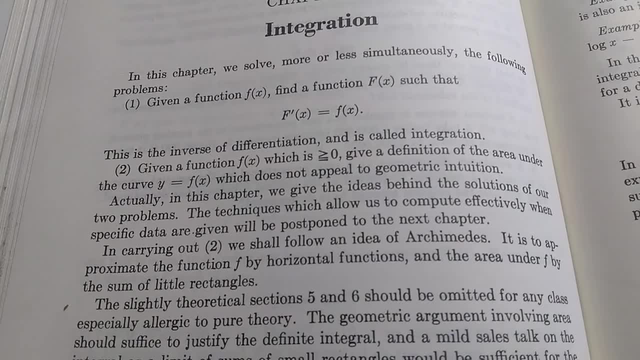 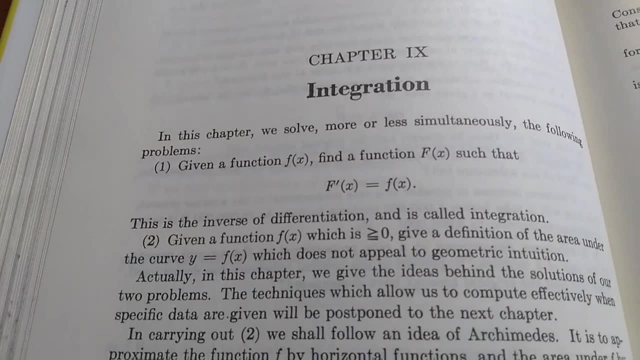 was the smell. I wish you could smell it with me. That's the nice thing about old books: They just smell so good. If there was some way to transmit the smell through you to this video, I would totally do that. Thank you. 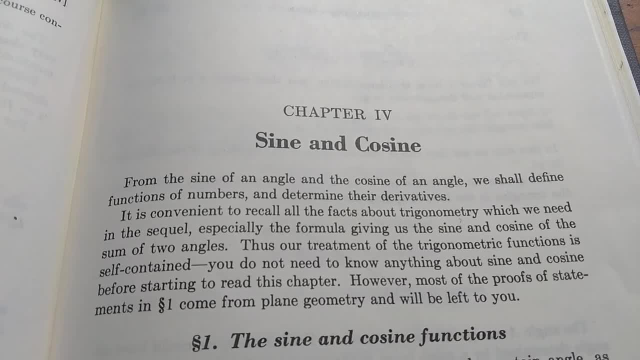 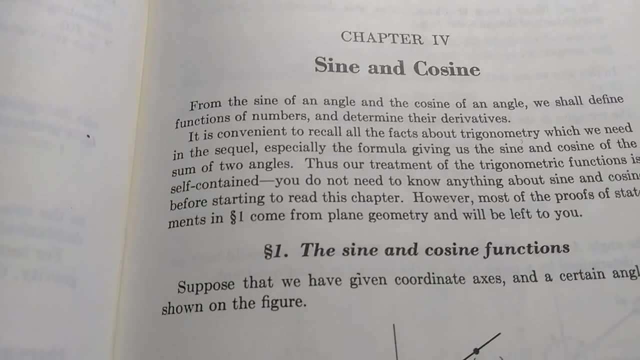 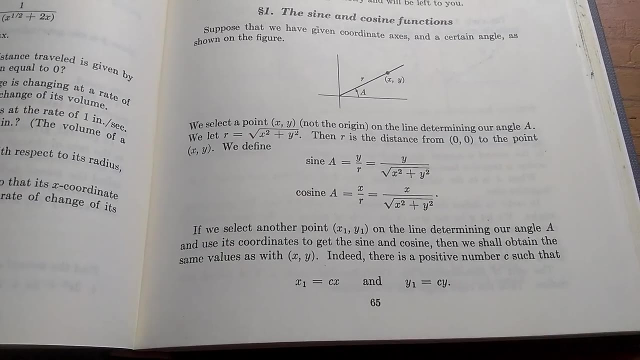 This is a very interesting chapter. It's the chapter on sine and cosine, and he starts off by just defining the sine and cosine from scratch, which is kind of nice. I often find that when people take calculus they forget a lot of the 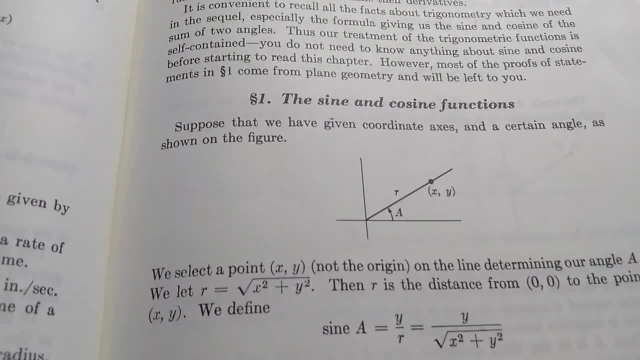 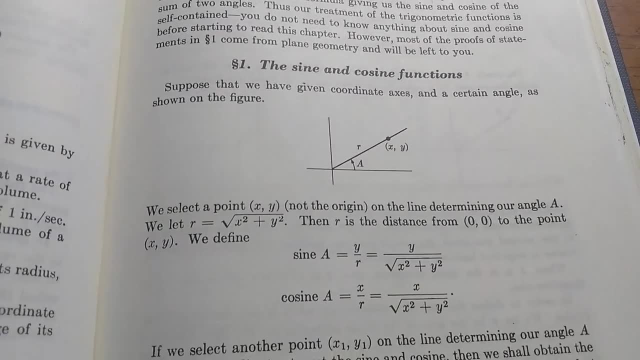 trigonometry, and that's normal and I honestly think it's expected. Learning trig is pretty tough and we tend to forget things. We're human. So he defines sine and cosine. Let's keep looking, Let's just skim through this together. Yeah, he just keeps going on and on defining. 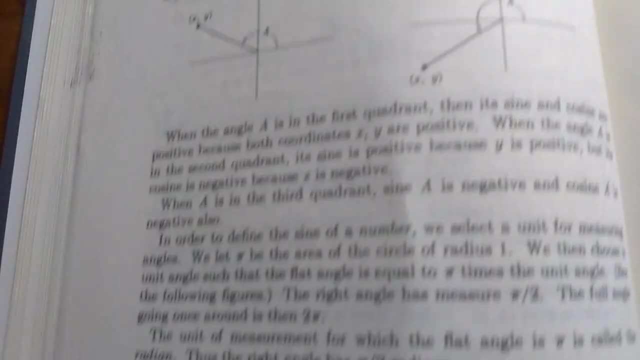 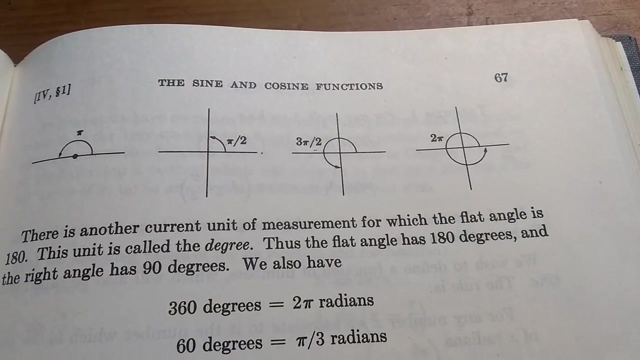 everything. just reviewing all of trig, at least the important stuff, I like how he emphasizes the quadrantal angles here right Pi, pi over 2,, 3pi over 2, and 2pi, And he gives pictures of each. I mean these are probably some of the most. 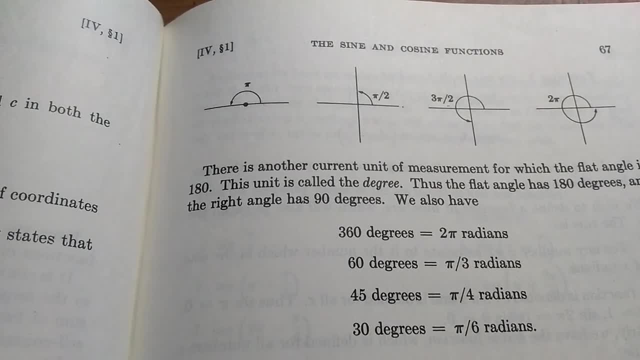 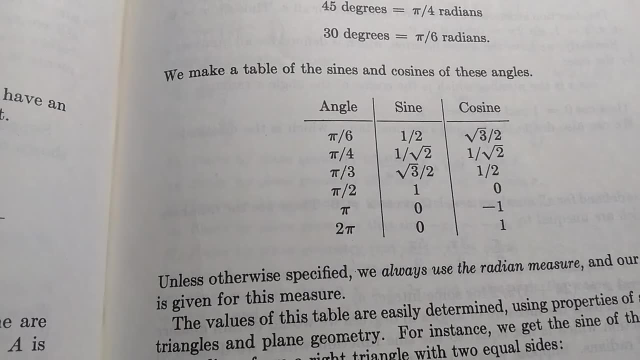 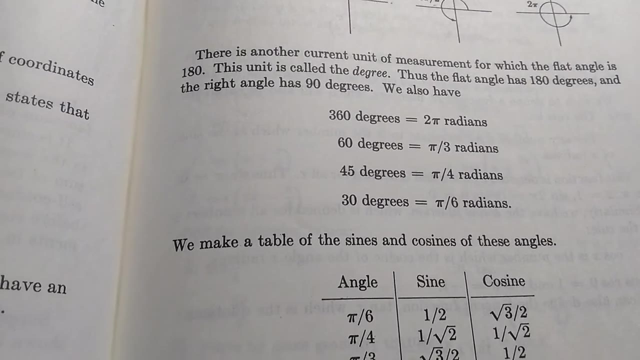 useful common angles that come up in calculus. He gives their measures in degrees and then he has a little table with the other important values. These are the values of the sine and cosine which people always tend to forget, and I guess that was true even back in the 60s. right, This book was written in the 60s. 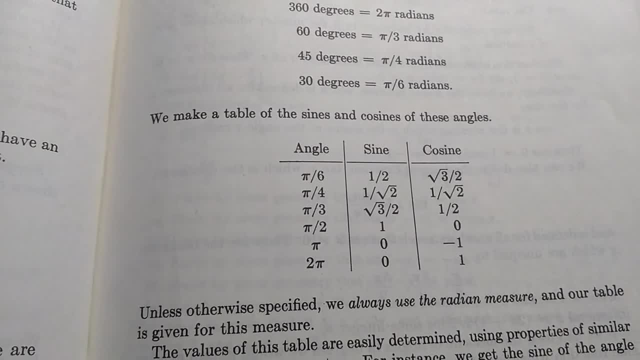 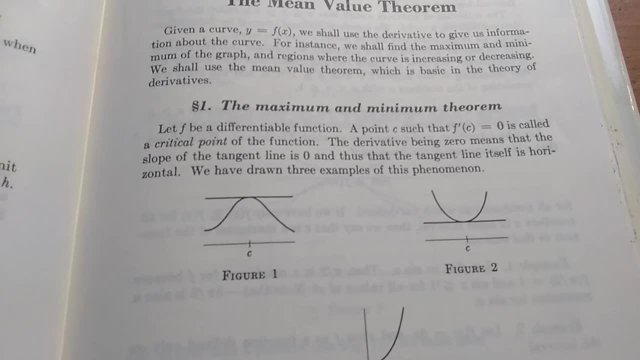 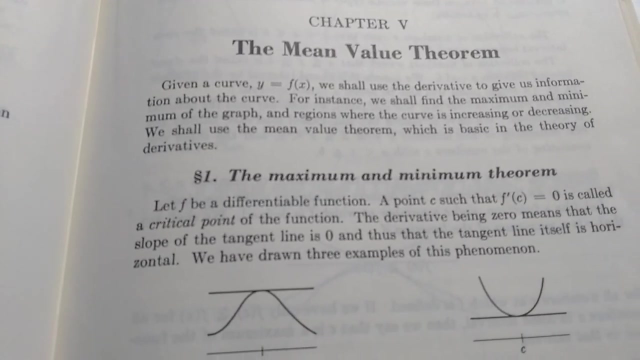 and Lange knew that people struggled with this, so he decided to put this in his calculus book. The writing in this book is absolutely phenomenal from a mathematics point of view. This is the chapter on the mean value theorem, and then here he talks about critical points and he gives some examples of 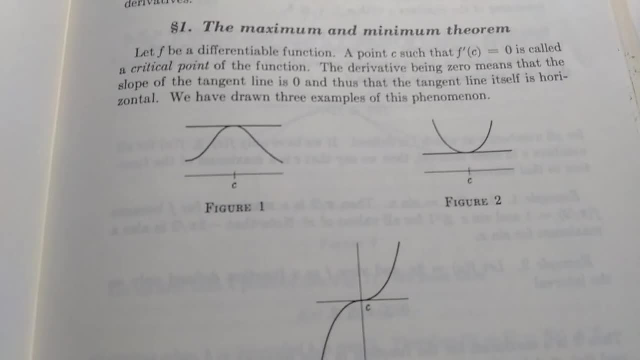 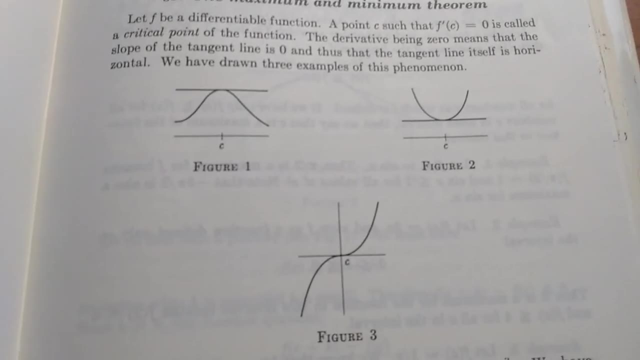 pictures. And this is exactly what I do when I teach calculus 1. I give examples and I also give the functions and I try to give all the possible cases so people really understand what is going on. And Lange does the same thing. Fabulous book. 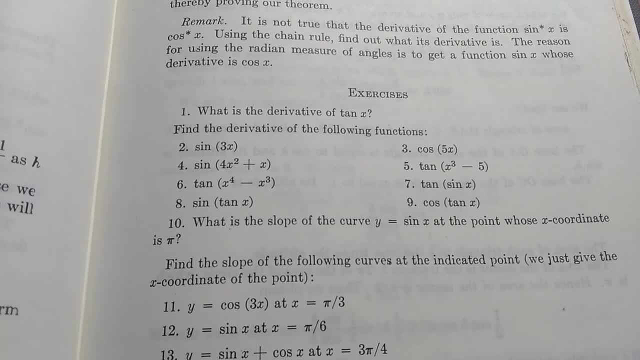 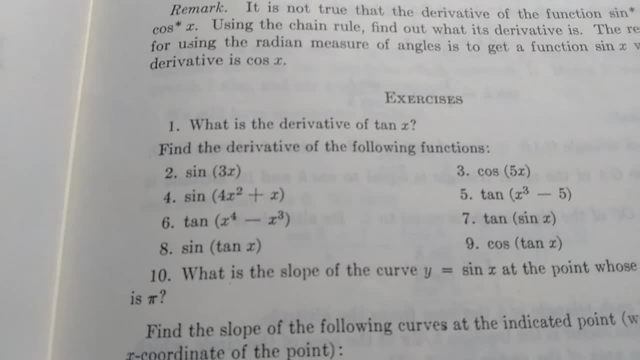 extremely, extremely well written. So this is the section on derivatives for sine and cosine And you notice the problems are not too bad. It's not too difficult. He doesn't go nuts. Looks like there's a lot of chain rule examples. 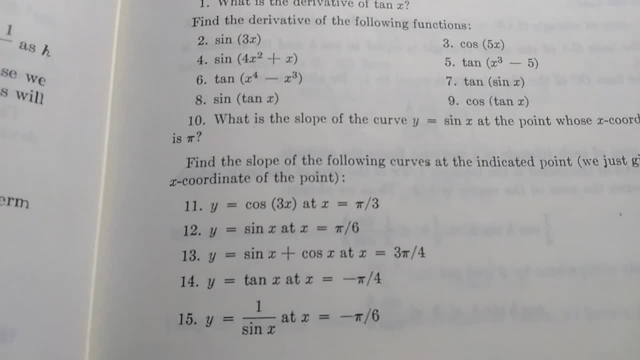 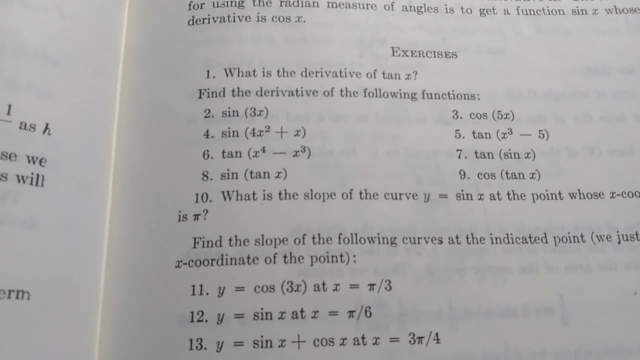 Here. And that's it, Only 15 exercises in this little subsection here. So not bad, which is kind of nice, right? You read the book. There are short little sections and then you do the exercises. It makes you feel accomplished. It makes 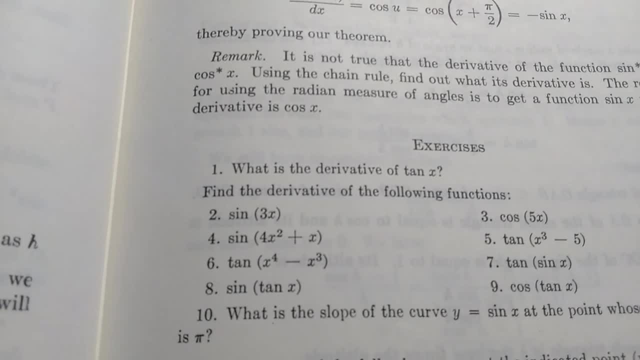 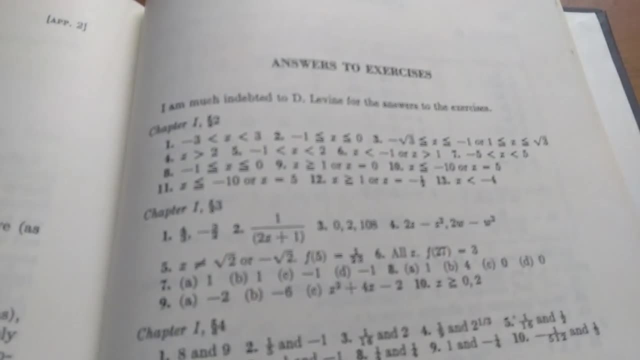 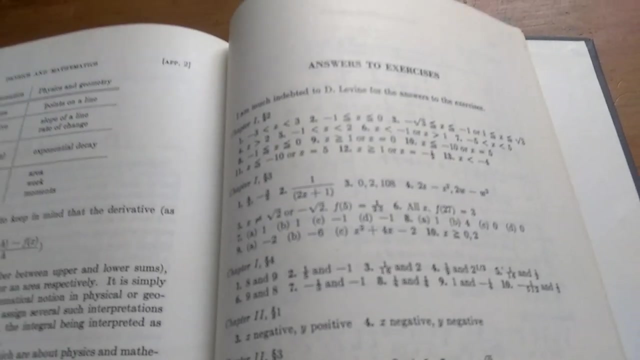 you feel good and you basically learn. You learn a lot of mathematics by reading this book. This book provides answers to almost all of the exercises, which makes it an excellent study. This is a great book for self-study and it's a great book to read The way it's.